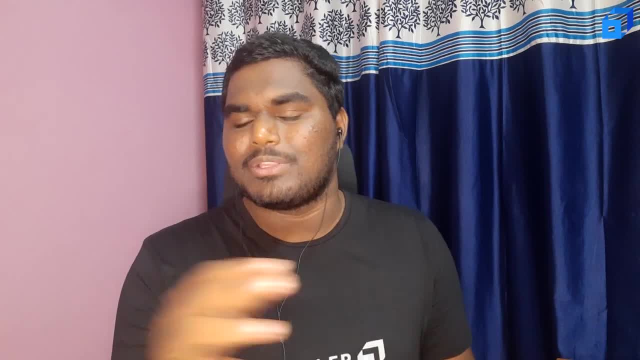 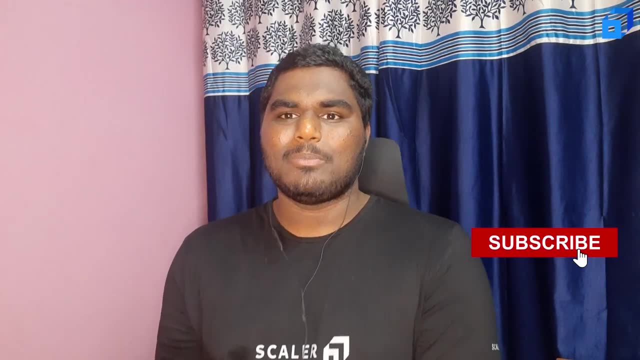 works and what are all the things that involves in client server architecture. So, without wasting any time, let's get started. So before starting, so if you are visiting channel for the first time, don't forget to subscribe. If you like the content, please hit that like button up, If you have any. 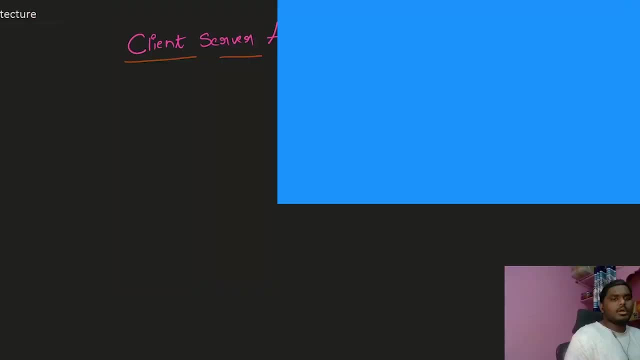 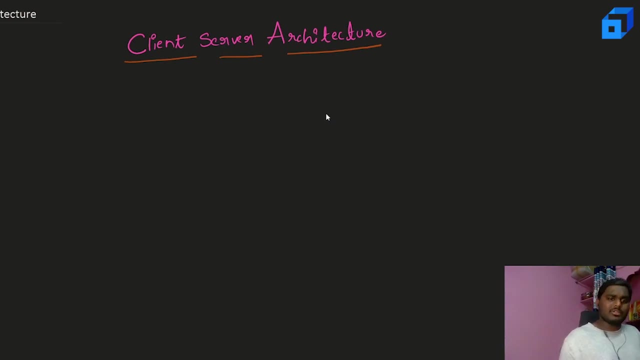 queries or questions, please let us know in the comment section. So let's start discussing about a client server architecture. So before jumping into the discussing about architecture, first we will see what are the terminologies, So what is meant by client. So client might be user. So simply I will tell you with one example for better understanding. So one server. 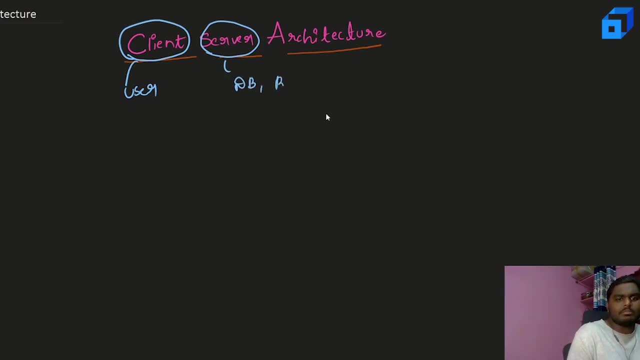 might be some database or some backend thing, So you can consider client as working at frontend. So let's same. let's say okay. let's take an example of codechef. okay, so i have an codechef website. okay, so i have logged into using my credentials and there will be something for our search with. 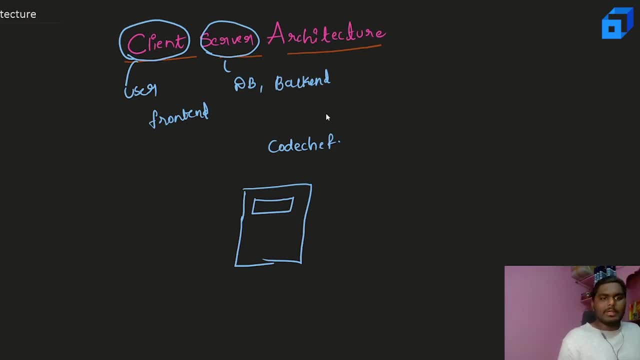 username. okay, so i want to know what are the ratings of my friend. okay, so i will provide his particular username right now. so what i will get? i will get all the details of his ratings and what are the context, histories and all. so what exactly happens behind this thing? okay, so whenever you 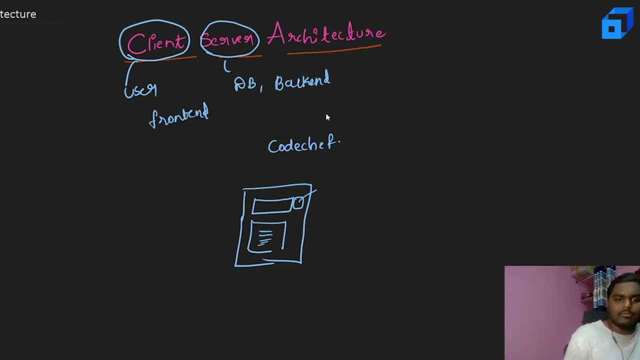 hit that submit button or search button so it will go to a server. okay, you can typically call this a backend, so let's assume there are some db over there. okay, which which is storing all the information of codechef users. okay, so whenever you search for with that particular username, it will return you the details of the that particular user. okay so. 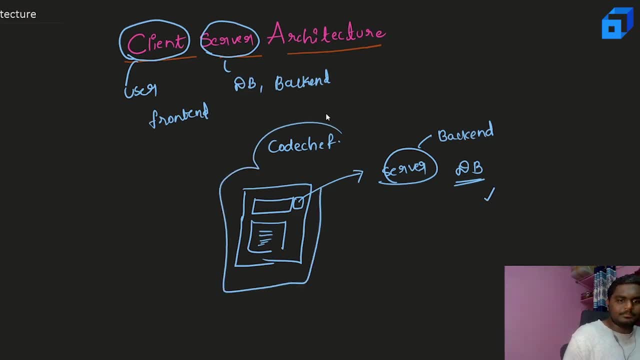 here. this particular, like the web application which are using to send an request, is called as a client side. client side which you are using directly, and this particular part you are you. you have all the additional details. okay, so we are gonna let this see Chef ceux diretly, and this particular part you are using. 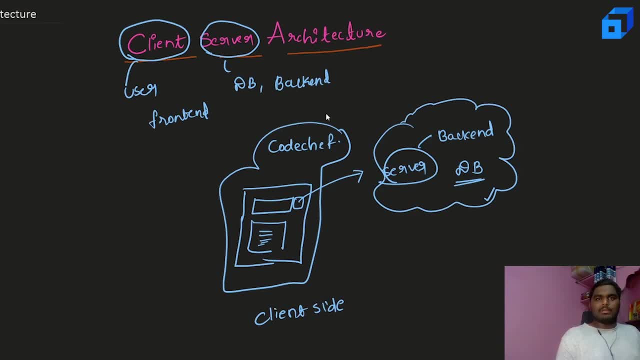 using this particular Part. you are using those like for upv, Oh, the details of coaches which we can indirectly, you don't know, like someone who is an 12th standard or 10th standard guy came, honey searching something on Google. okay, he don't know exactly what. 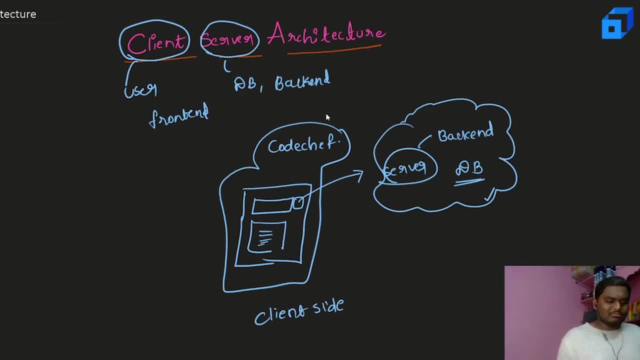 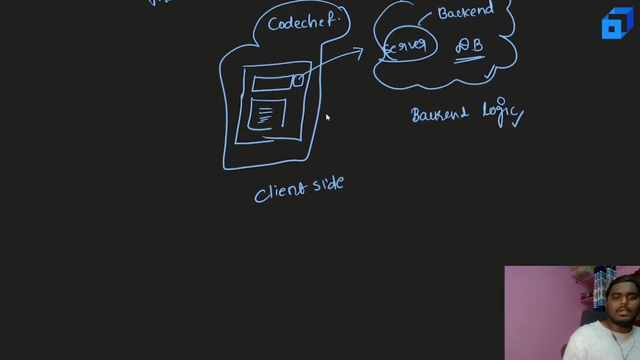 is happening behind that. he knows something like: if I enter like something, I will get something. that's it. okay. so this is the back-end, so back-end logic, kind of stuff. okay, so this is in simple. what is client and server? okay, we come to more details later. okay, first we'll discuss what is a before client server. 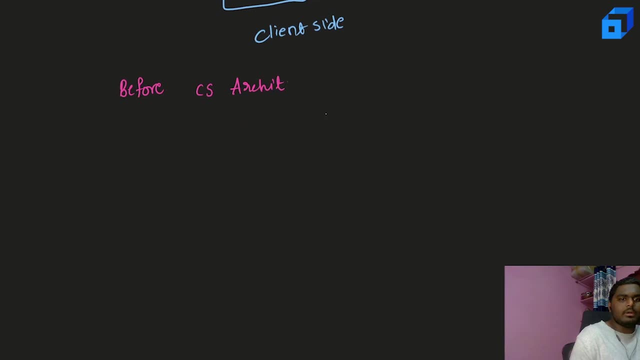 architecture before client server architecture. so before this we used to have mainframe computers. you can call them as a standalone systems. what does it mean? so let's say you have a one computer, you have one computer and you have created some database by using any SQL SQL database. okay, on your local mission. okay, so this? 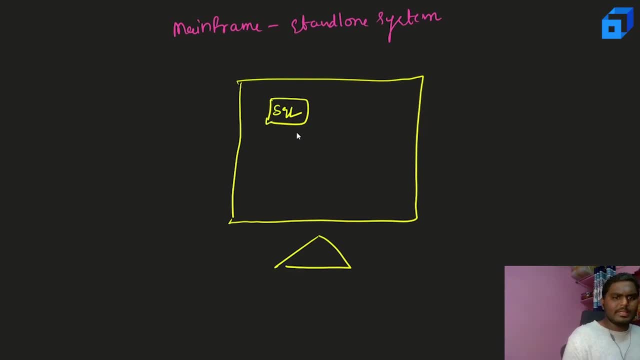 is your system okay. so there is some sequel database we have created with some tables and all, and also you have created one, a web page to access the sequel data, okay, database. so can I ask few questions here? now it is in your system, so can your friend. 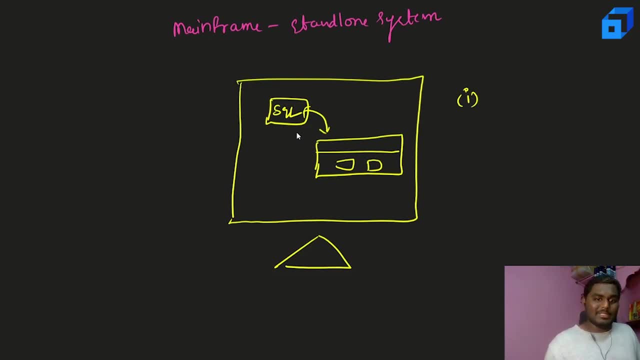 able to access that data, which is residing on the database, from his own system without having any connection? no, it is not possible, right? so that kind of systems are called as an standalone systems, where the data has been restricted to one particular system. so you might be the client and you are the owner. okay, server is residing in your. 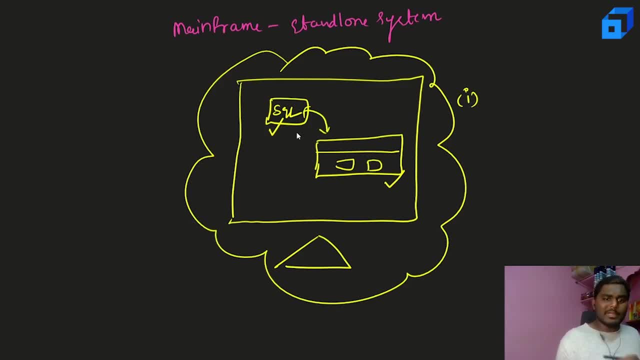 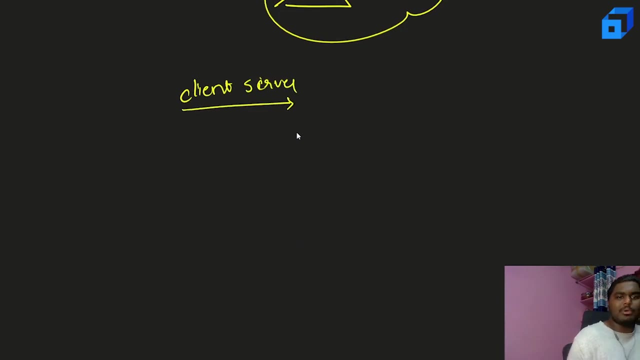 mission itself. okay, so others are not allowed to use that particular server. okay, so that is the before, before our client server architecture came into exist. now let's see what is a client server architecture? it is not new. okay, hope we have discussed this in while telling the. 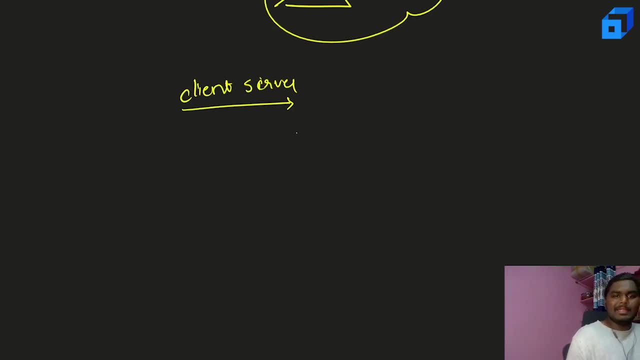 terminologies of client and server. so let's see in detail. okay. so basically, let's say you're at a client side and you will make some a request. okay, you will make some a request to the a server. what is a request? so a request can be anything, let's say, but wwwgooglecom can be one. 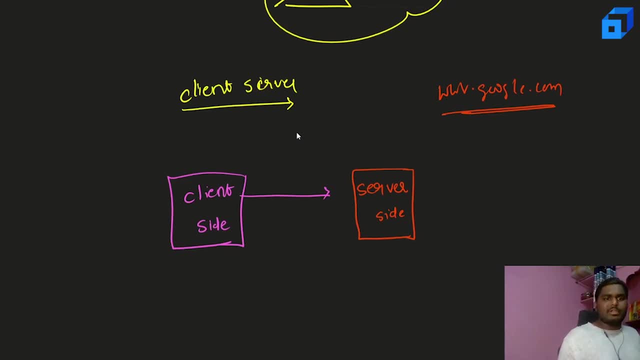 request, right, as I said earlier, searching with, like entering one- you a coach, a user name and I have expecting some, all the details of that particular user. so here the request is. so, such, with this particular user name, I want all the details. so there is one request, right? so 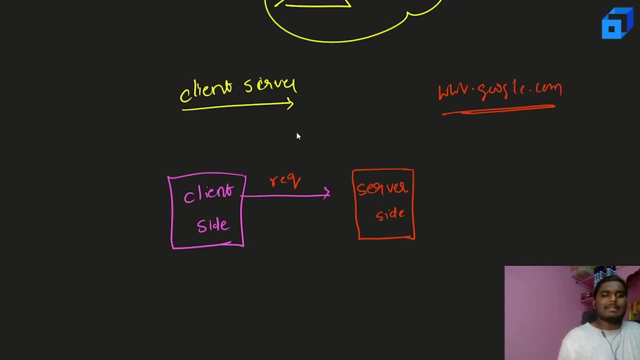 this is a request. so what is this server side content? so it contains some DB, like databases. so tell me, is that always? and data? is that always? and data? no, I don't think. so what might be? so it might be some calculations, logicals. let's say you are using an EMI calculator: applications, EMI calculator. 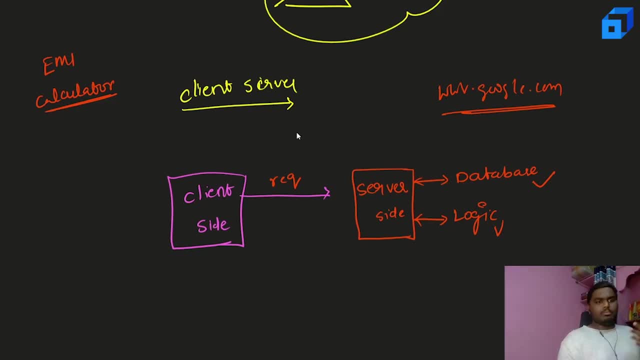 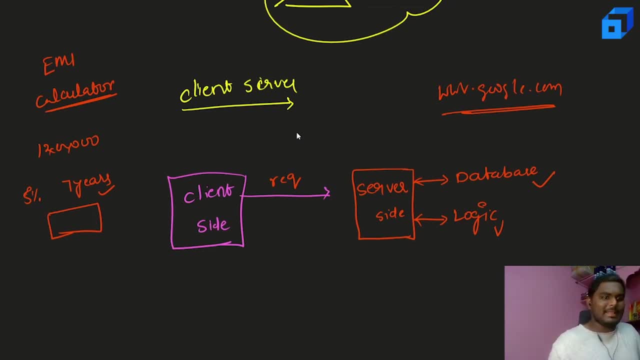 think is there any DB involved here? no, but still it's a request, right, so I can say that there is a logic as well. so in server said, in server said, I can say that both a DB and logic has been residing in particular mission. so here after like whatever, if you have such a with user of coach, of 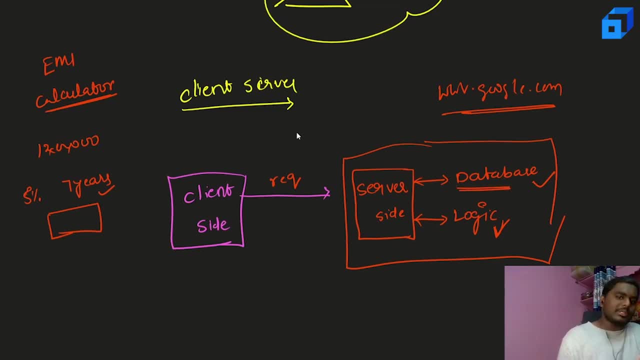 username, it will go to database and it has to return something to the client, right? so it has to return the details of that particular user, so it will send some responses back to the client, okay, so, even if it is an logic side, I like for this particular example, she'll dash to send some responses, right? so you have to. 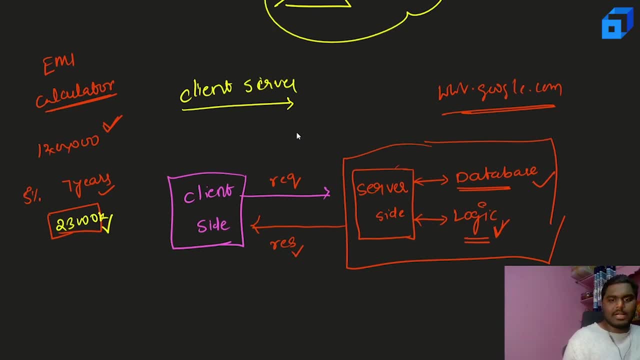 pay monthly twenty, twenty, three thousand kind of stuff. so even that is also an on a response. so this is how the actual account server look. architecture looks like, and we oftenly call this as an two-tier architecture to type architecture. so why today? so is there anything apart from a client side and server side? no, there is. 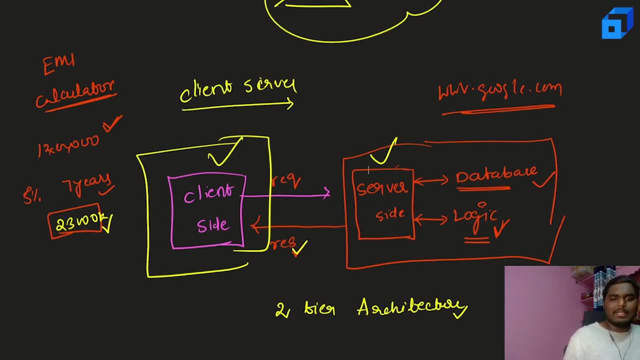 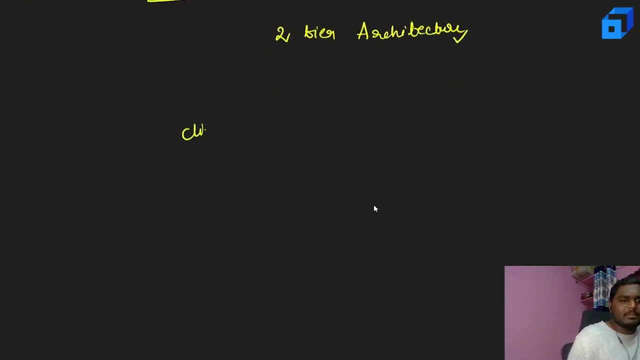 no other things involved. okay, now let's see few things which were involved. other things as well. okay, let say so. I have a client side and I have a like. I am dividing the server side into the two parts: okay, logical and DB. I know that sometimes I need not to go to DB, okay, so I'm pretty much sure that I. 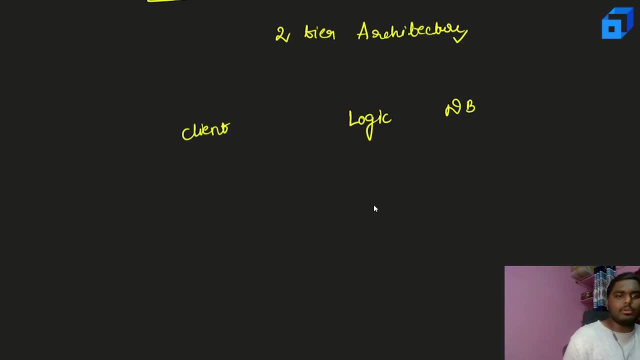 don't have a work with a DB always, so what I will do? so I will go to simply to logic and I will check whether it's a logical based out. it requires DB. okay, I will go to logic and I will check whether it's a logical based out. it requires DB. so 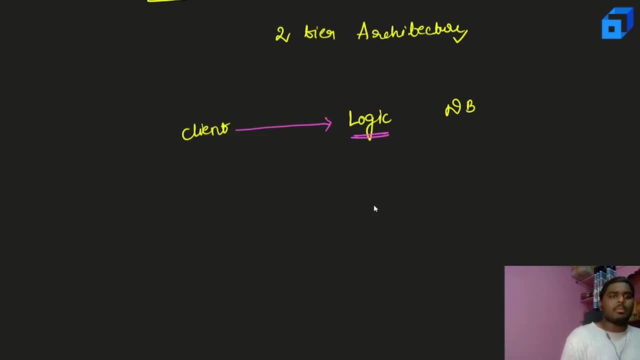 So if it is a logical based, what I will do, I will solve the problem here itself, ok. If it is an a logic based- sorry, DB involved, I would go here, ok. So this kind of things being called as a three tier architecture. 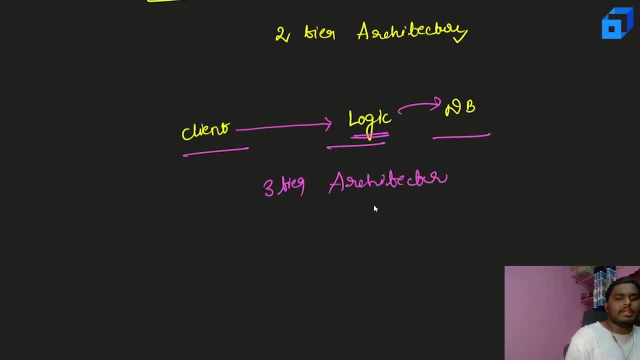 So one, two, three, three tier, So there is something like a entire architecture as well, entire architecture. What does it mean? So let's say you have a client and you are using some load balancers to process your request to different servers. ok, 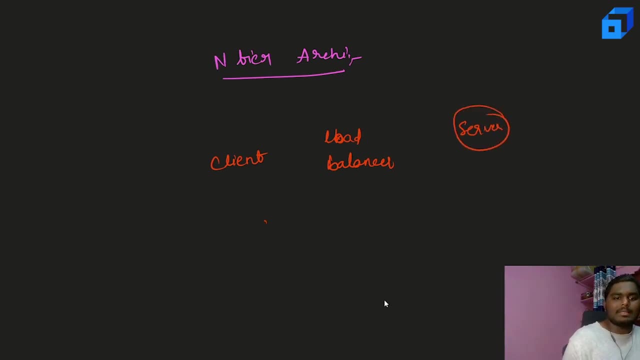 So let's say you might have one server but there might exist of different clients. ok, So, n number of clients, no guarantee right always. So do you think only one person can at a time can search in and google? No, Ok, So many people, some billions of people, used to search at a time. 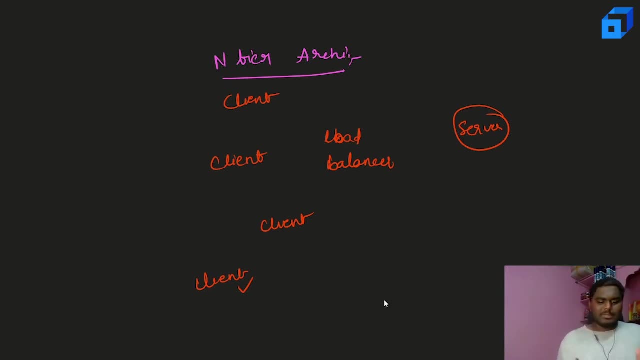 So how they are processing your request is So if they have multiple servers, they will use load balancers to divide your request to and process your request to multiple servers at a time to feel that you are in and, like you are the alone, you are using that particular system. ok, 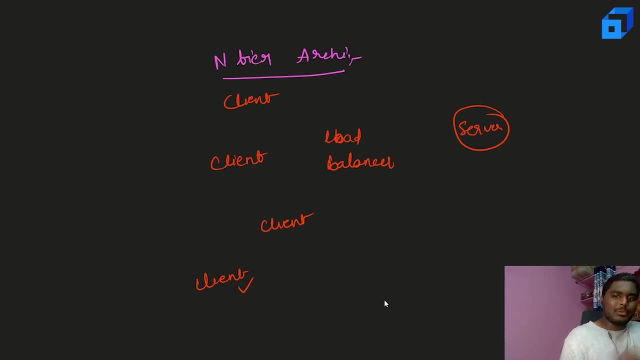 So and like so, instead of going to directly to the server. Let's say you have a cache. Let's say you have a cache, You have a cache memory. What I will do for the first time I will request. ok, So it will process to the server like it will go to the first, go to the cache memory and 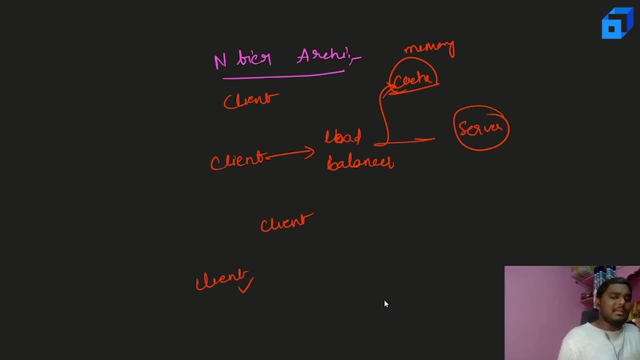 it will search whether whatever I have requested is there in cache memory or not. ok, So if it is presented, if it is there in cache memory, it will simply return from cache memory itself. ok, It won't go to the server just because of the fact that I have phone. ok, 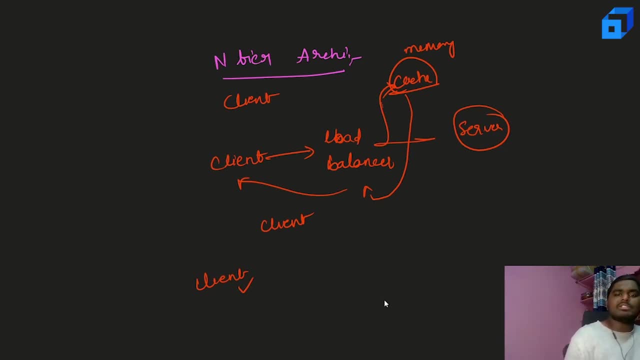 I have response for your request. So if it is not there in cache, what it will do? it will go to server and it will take that response instead of going directly to the client. It will go to a cache- first cache memory- and it will put a replica or copy of that response. 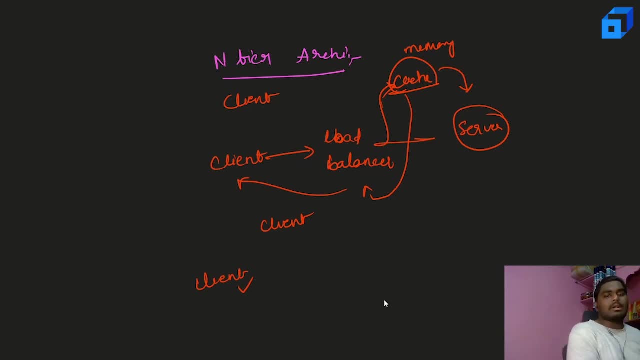 in a cache memory. Then it will return to client. ok, So here this like this. So we are. I have simply used a load balancers and cache here, So there might be other things will also exist while designing complex systems. ok, So in that situations you can call it as entire architecture. ok, yeah. 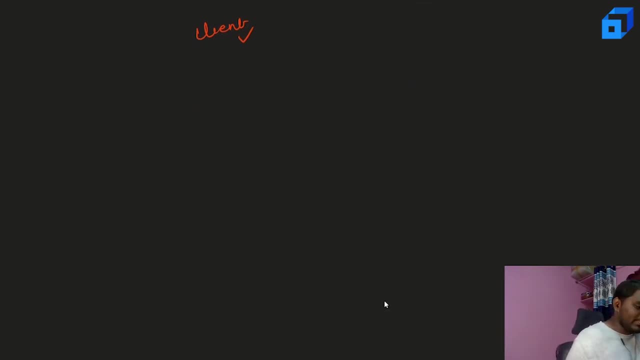 So, yeah, let's move on. So the next part is thick clients. Clients have been divided into a thick clients and thin clients. What are they? Who are they? Right? You might have that question. Let's see. So a thick client is, or something. ok, 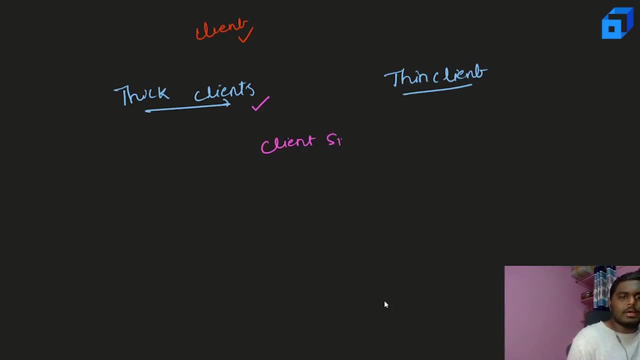 Let's say, hope you have a no client side rendering and a server side rendering, server side rendering. What does it mean? So, basically, So do you think all the calculations you do will go to the server? No, let's say, I have simply developed an calculator app. calculator app- ok. 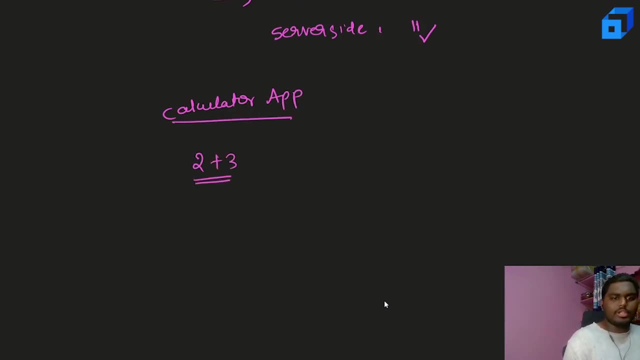 So I will enter two values, Two plus three. ok, Do you think it will go to the server and it will do some logic and it will come back to a result? No, So I can handle this in my code base only, like at the client side as well.